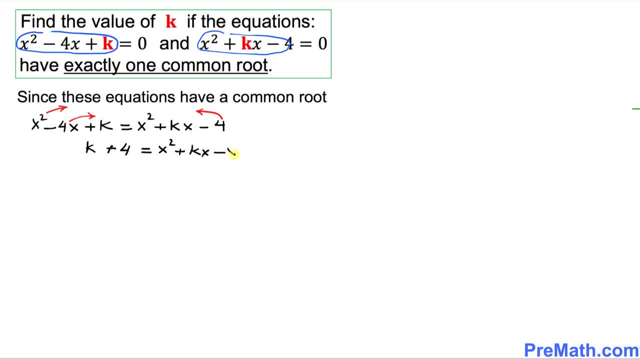 and this: when you move this negative x, positive x square become negative x square and negative 4x become positive 4x. Now in our next step, we can see that that this negative x square, positive x square, this cancels out. so we simply have k plus. 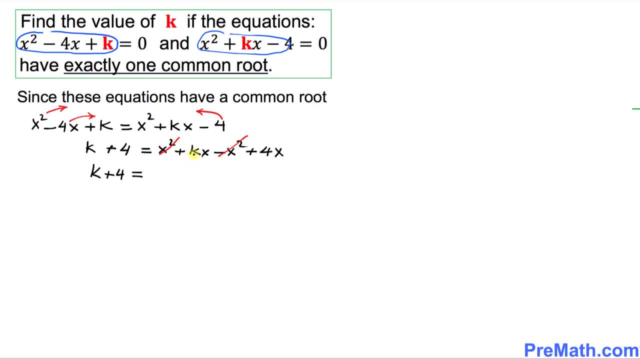 4 on the left hand side equals to over here. I can simply factor x out. If I factor x out, I got k plus 4.. And now I can divide both side by k plus 4 and k plus 4 to isolate x. so simply, this is: 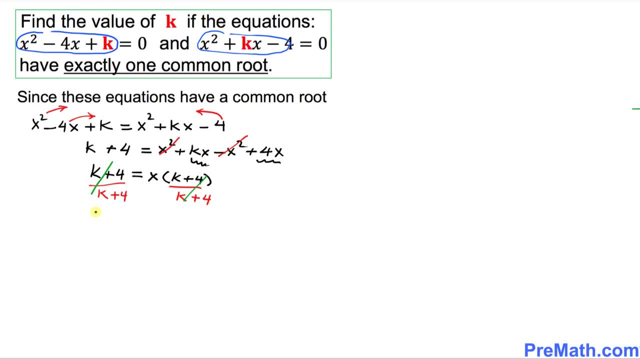 gone. this is gone. so we got x equals to 1 value. And now the very first equation. I am going to call it equation number 1 and I am going to substitute it. I am going to put this x equal to 1 value in that one. so wherever you see, this is by: 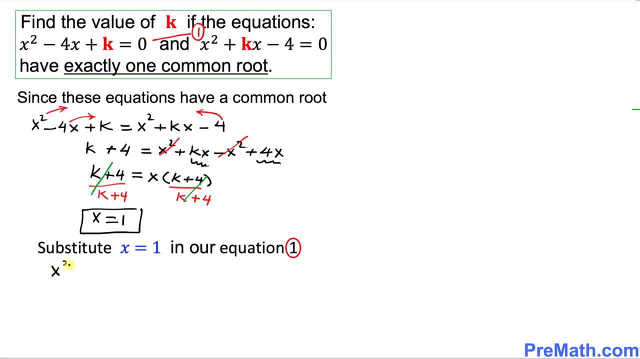 the way this is x square minus 4x plus k, equal to 0.. So what I am going to do is I am going to replace x equal to 1 value, so this is going to become 1 square negative 4 times 1.. 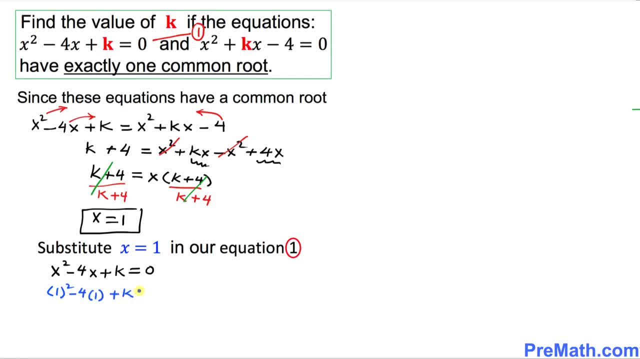 Ok, 1 plus k equal to 0. so that is going to give you 1 square equals to 1 minus 4 times 1 is 4 plus k equal to 0. this become negative. 3 plus k equal to 0 means we got k equal to. 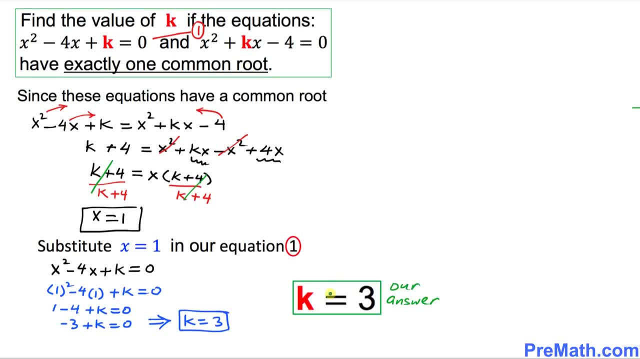 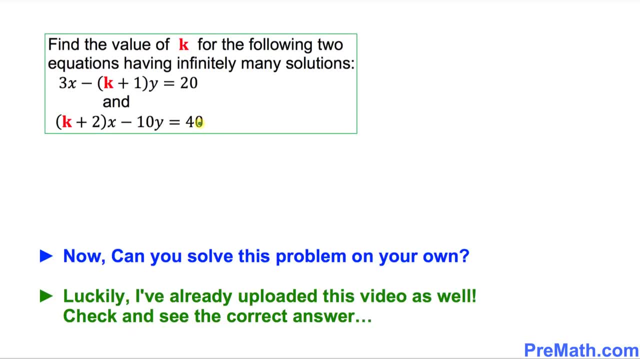 3.. So that's k equal to 3., 2., 2., 3. and it turns out to be our answer. And finally, here is your assignment. can you do this problem on your own? you can take your time.